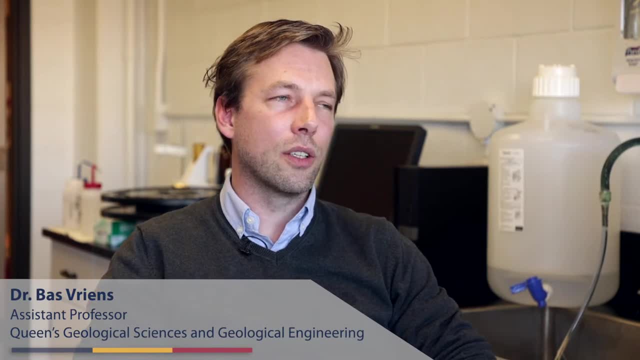 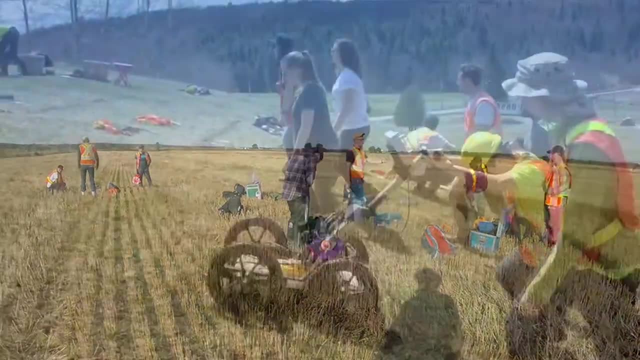 We're a relatively small department but lots of things going on, So a lot of activities organized by students- field trips, career events- So it's a very open door, supportive environment that I feel as a faculty but that the students enjoy. 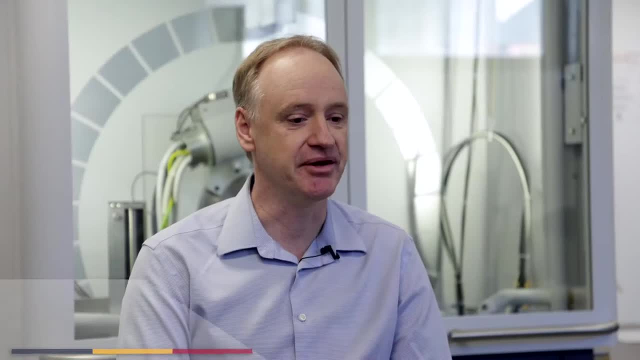 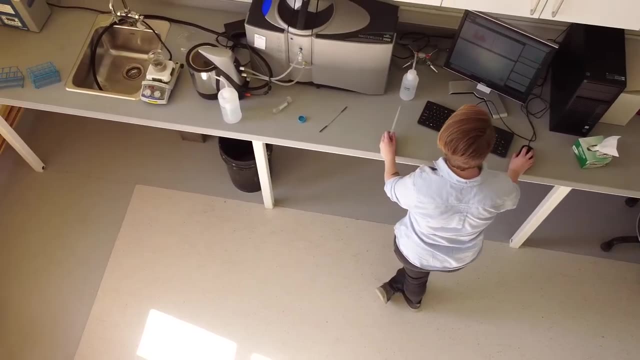 I feel as well. I think It's a very diverse group. We're one of the only geoscience departments in Canada that has parity in terms of gender. When I was applying to programs, I would immediately look at the list of people in the department. 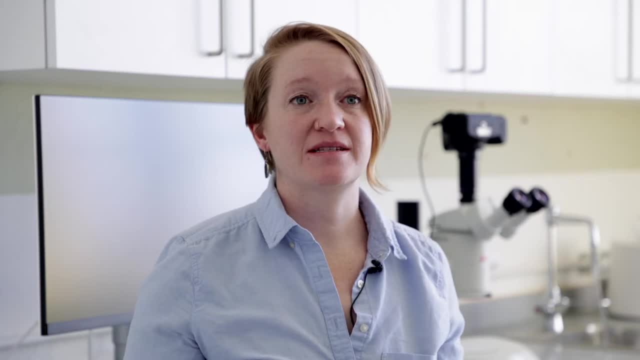 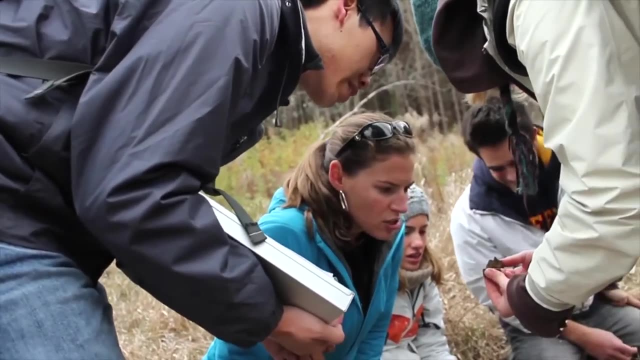 and one of the things that really stood out to me about Queen's was the gender diversity that our department has. We've got a number of initiatives that are going on in our department to make sure that we are diverse not just in gender but in all aspects of diversity. 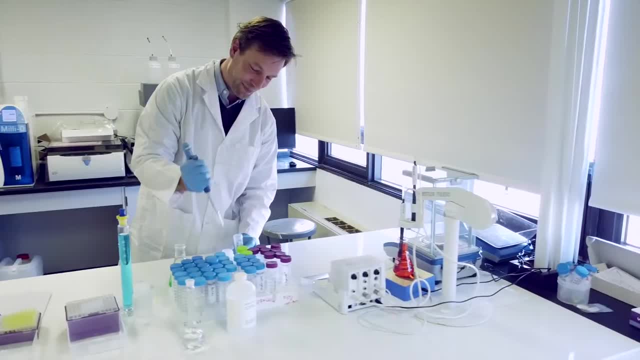 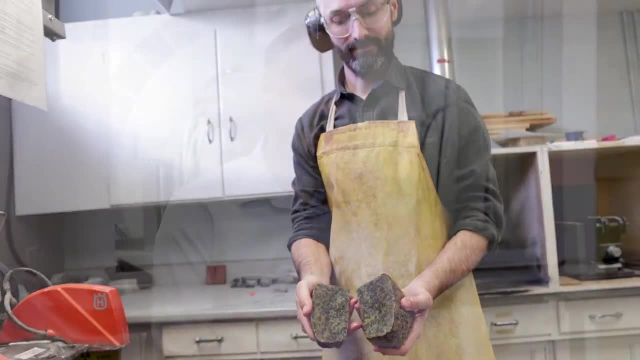 We have researchers that are the best in their field- whether it's in geochemistry, whether it's in geophysics or whether it's in traditional geology- And we have a very hands-on policy with our students. It's not just upper-year graduate students that get to come into the lab and work. 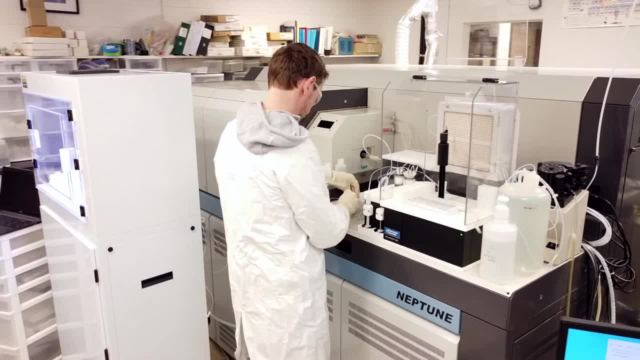 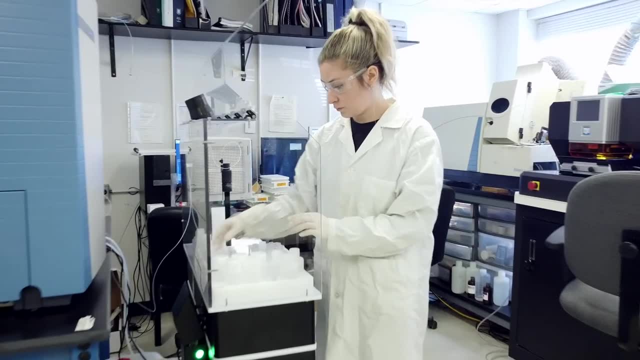 We involve our undergraduate students Some of the high-tech, state-of-the-art instruments that we have in our department. students receive training on that as well. Our students end up everywhere. We're working at mining companies or geotechnical engineering companies. 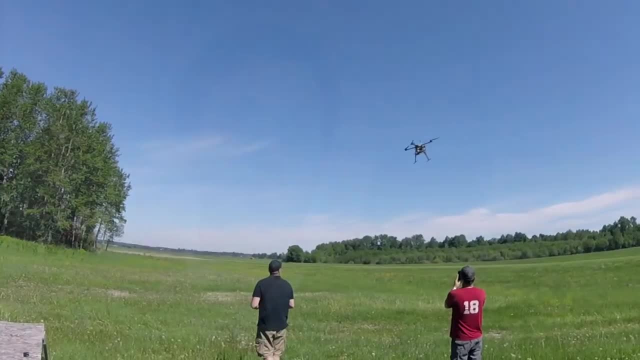 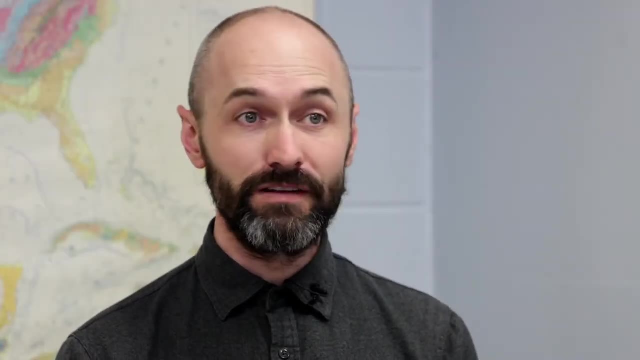 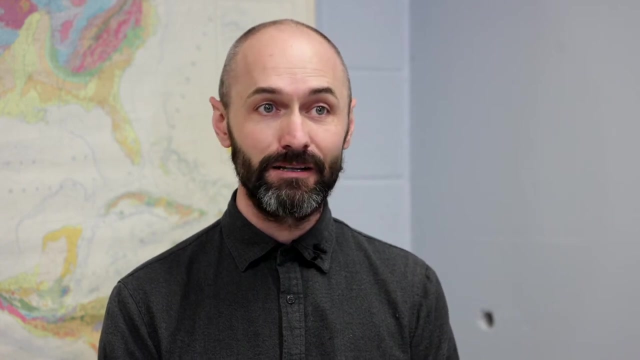 environmental consultancies, banks, reassurance companies, even data and IT companies. Humanity is facing a lot of interesting challenges that we've never faced before. Geology provides that link between humanity and the planets. We're going to be one of the first people that are going to be on the surface of Mars. 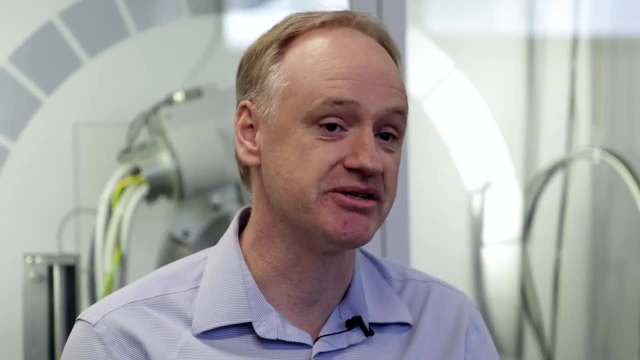 We're going to be some of the first people that come up with the answers to our climate questions. I don't think there's any better time to become a geoscientist or a geoengineer in Canada or globally. 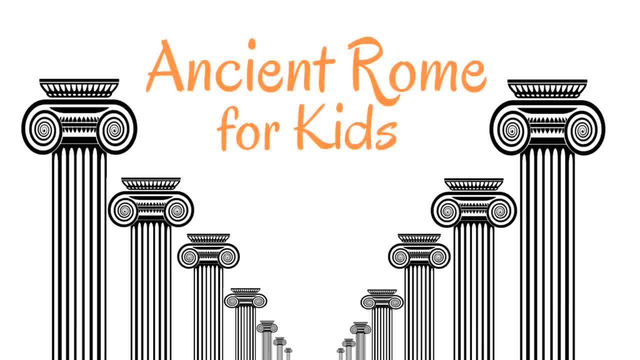 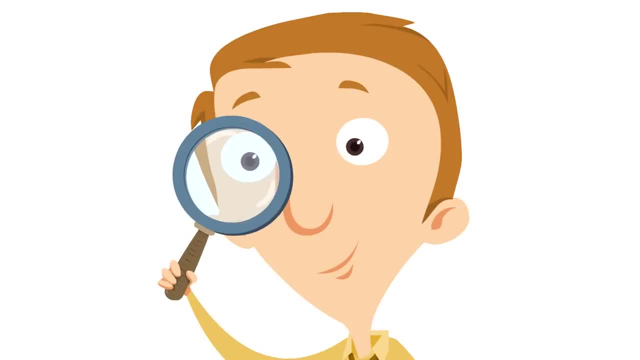 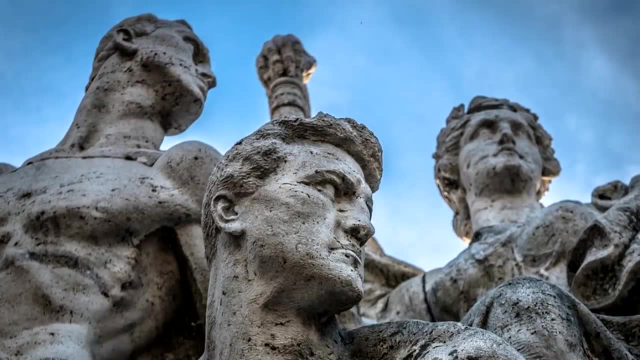 This video is all about ancient Rome- for kids or for just about anyone who wants to learn about this amazing ancient civilization that still influences us today. We are going to investigate and dig deep to give you the full scoop on this fascinating civilization. We are going to see our fair share of statues.